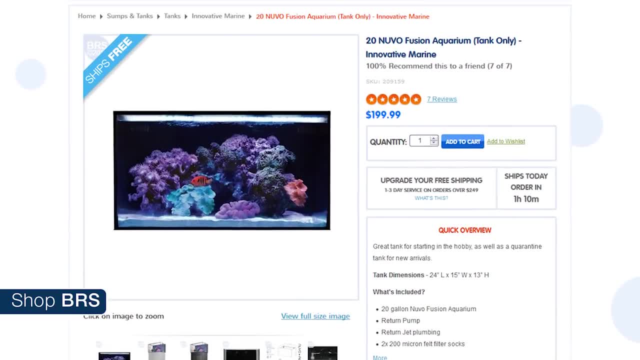 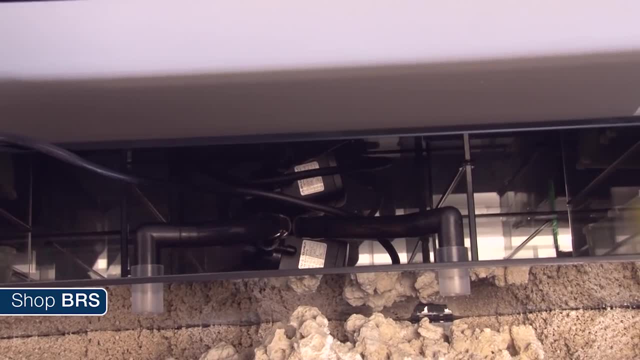 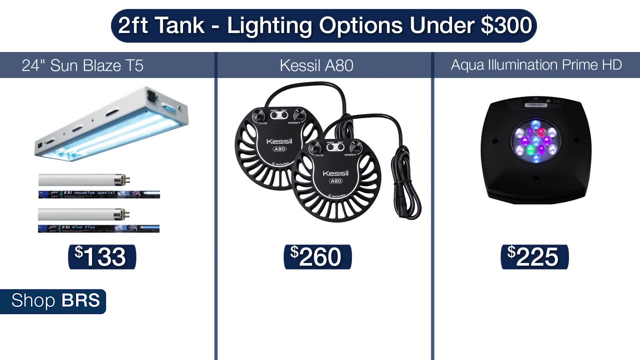 good example. The tank itself is more costly than an off the shelf tank. It is pretty popular for newer reefers. on a budget, I am going to try and keep the lighting option under $300 for a two foot tank. The lowest cost option will be T5's for sure. T5's will maintain a wide variety of corals and a simple 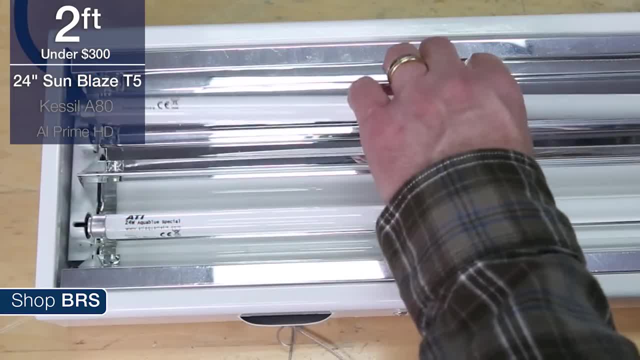 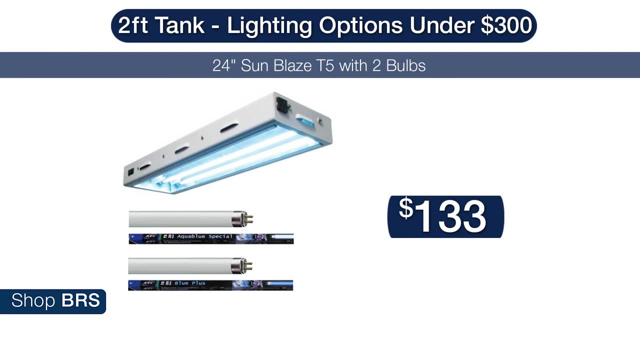 sun blaze tube bulb fixture is only $92.99.. Add a pair of T5 bulbs for another $40.. Likely one ATI blue plus and one ATI aqua blue special. That is only $133 for a solid reef tank lighting solution that is specialized as an even spring tank. 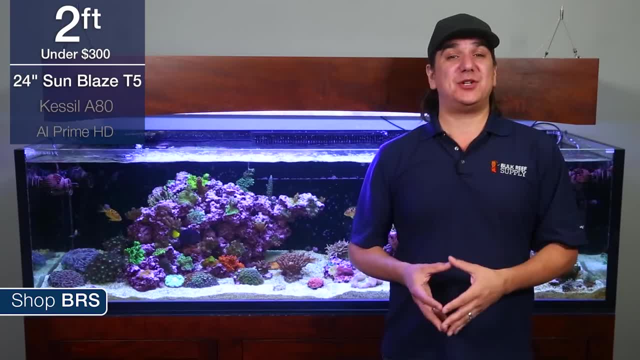 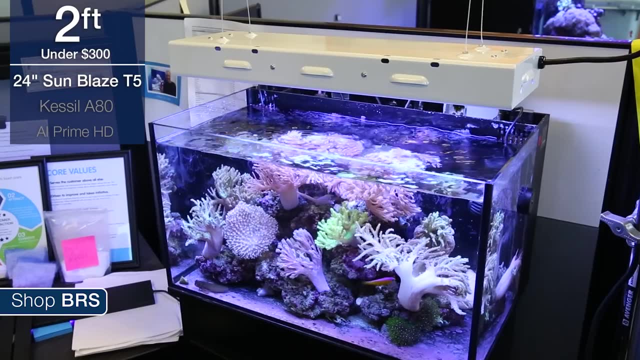 You might be tempted to get the four bulb option, which is about $70 more for the fixture and certainly an option particularly on deeper tanks, but not a requirement. You can keep a lot of corals healthy and happy under a tube bulb fixture. You will have to hang it. 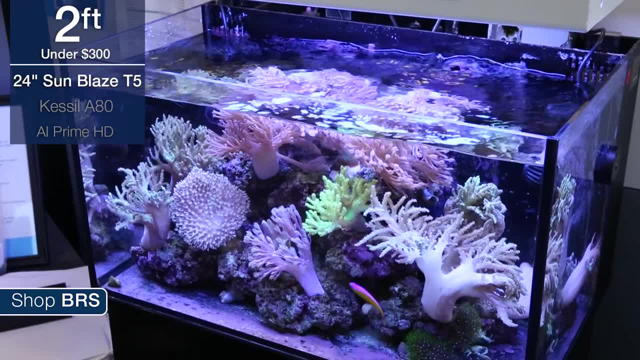 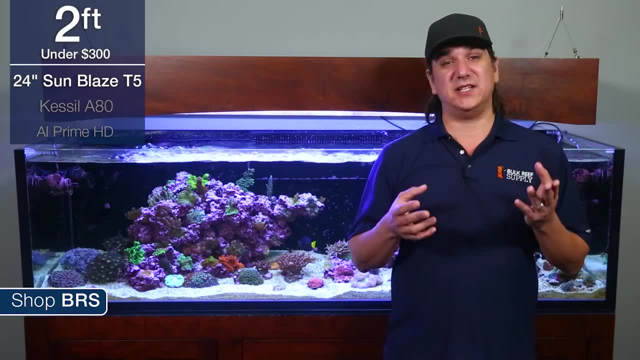 from the ceiling or some type of wall mount, like something you would get from a hardware store. I will note that the sun blaze is really designed for horticulture, which means it is particularly important to keep it away from salt spray to extend its useful life. However, at $93. 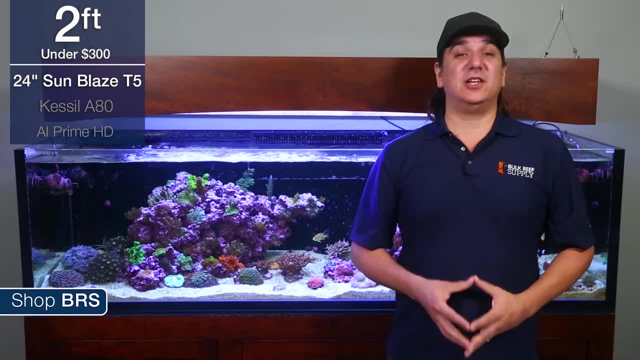 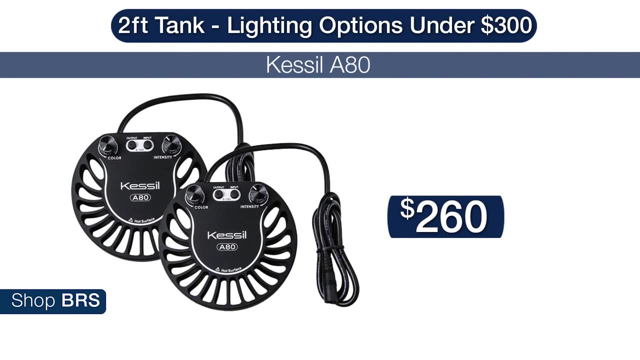 it is certainly the lowest cost option out there, Right after that, particularly on the shallower 2 foot tanks like the Nuvoo. one of the lowest cost options is a pair of the new Kessil A80's, which will run you $260 for a pair. The Kessils. 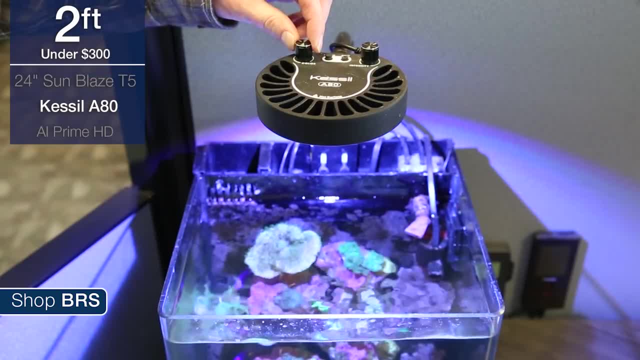 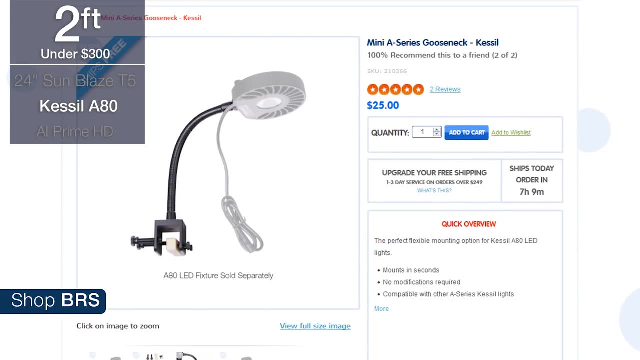 are an LED option which doubles the price but adds the color intensity and shimmer adjustability that LED's are known for. They are also low profile and have a mounting option arm available for those who want to hang it off the side of the tank. The two individual 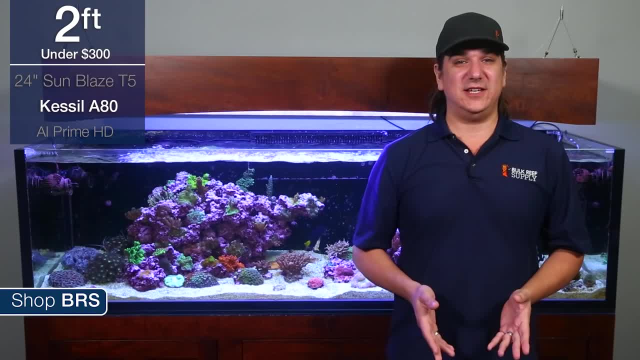 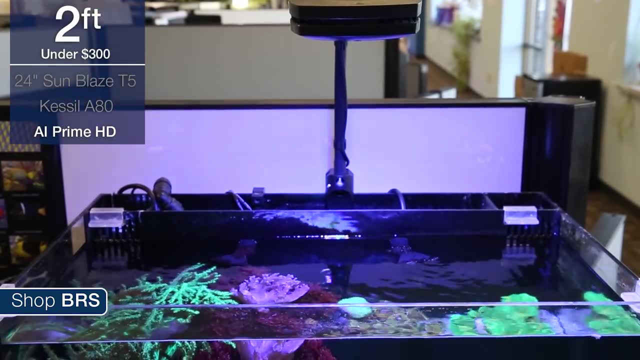 light sources will make aquascaping and evenly lighting the tank fairly easy. At $225, I would also consider a single AI prime HD. The single light source will obviously be brighter in the center and dimmer at the edges, but if you only keep low light corals on the edges, it might be perfect for a reef tank. 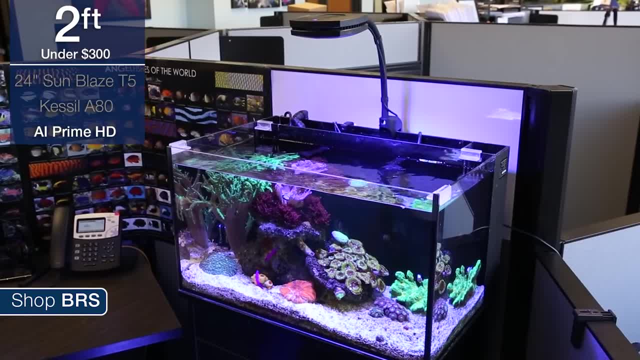 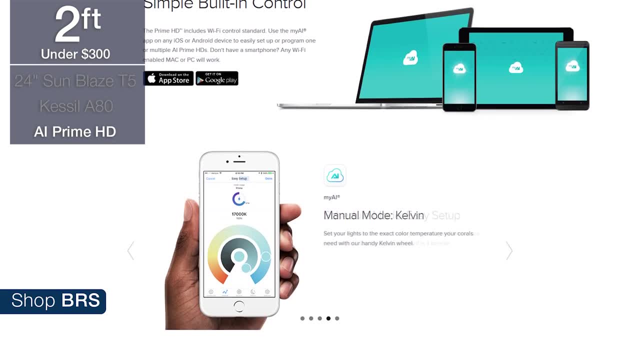 on a budget. However, the prime is also a very scalable option. If you end up wanting more light down the road, you can always add a second. prime AI is a trusted LED industry leader Only option at this price point, which is controllable via your phone and has a flex arm mounting. 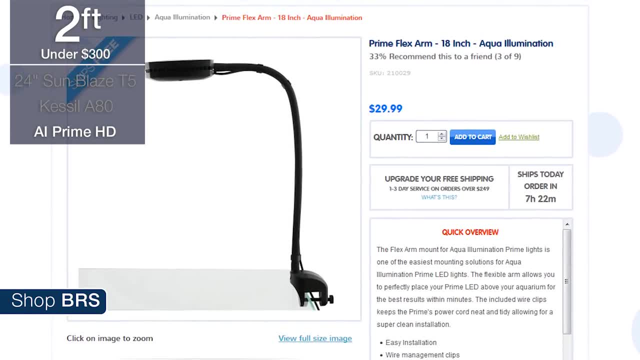 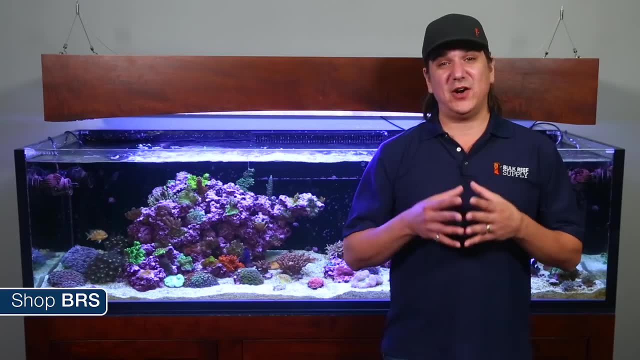 option available, which is a mounting option almost every reefer prefers on this size tank. On a 3 foot tank, I will focus on a 40 breeder, which is by far the most popular 3 foot reef tank and also very frequently goes on sale at Petco for $40, which is a great deal to take advantage. 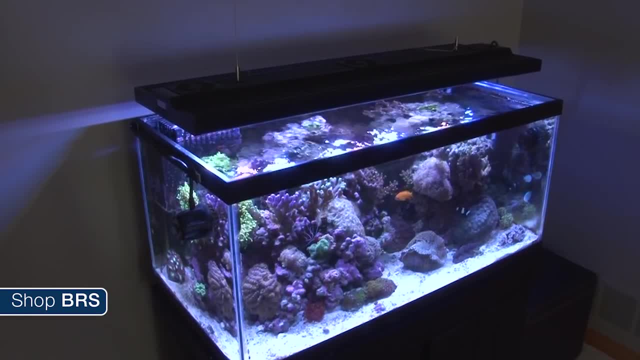 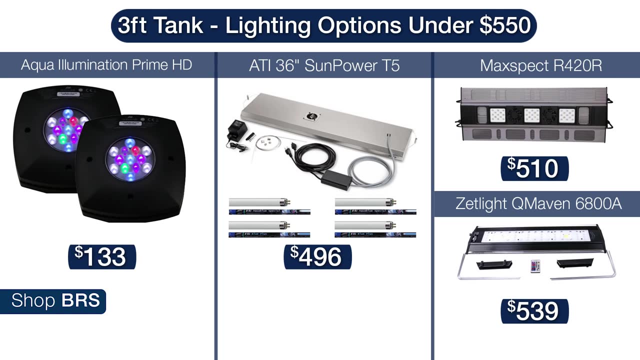 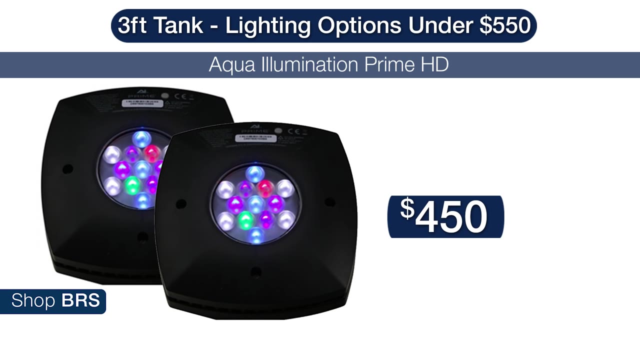 of That is good, because lighting options start to get significantly more expensive because it is almost required that you use an end to end fixture or multiple lights. at this point, Best I can do is provide four solid options under $550.. This time, I think two AI prime HD's are likely the best budget option out there at just $450.. 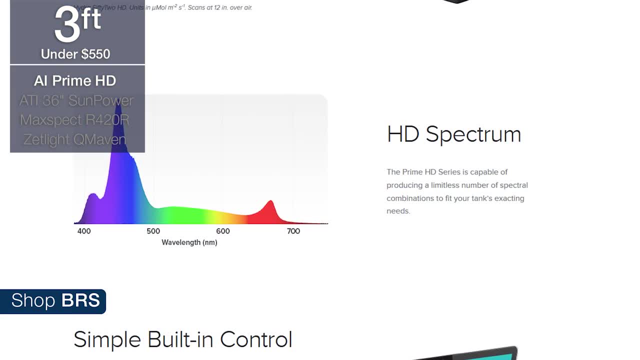 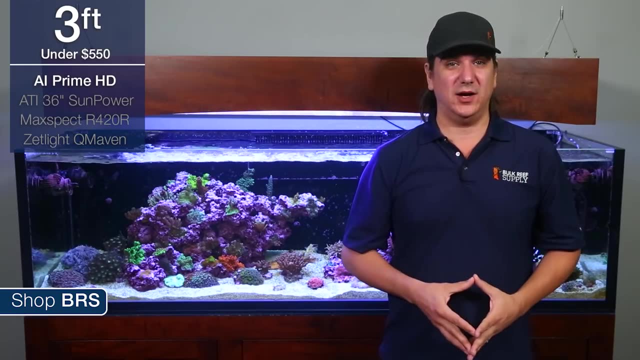 Again. they have all the awesome connectivity features and they are all great for light activity features. most people want All the popular LED spectrums. easy to mount and low profile design, but also at $450 are probably the best value option as well. Sunblaze doesn't make a 3 foot T5 version, so you have to step up to a 4 bulb ATI for. 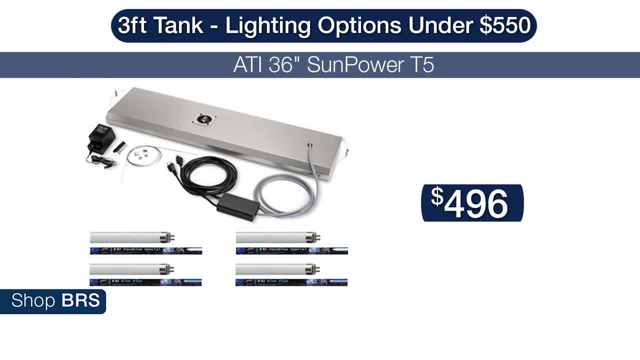 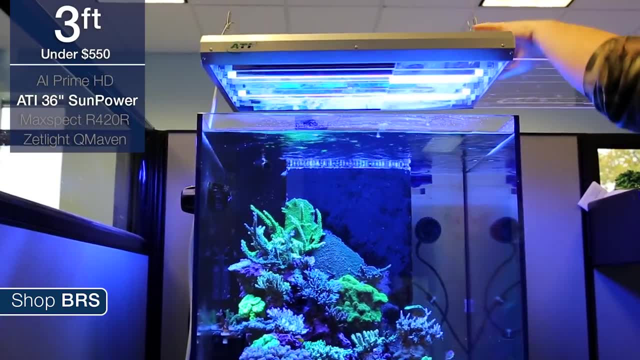 $416 plus $84 for 4 bulbs, so around $500.. However, you get a light design for a reef tank, active cooling, optimized reflectors, a splash shield and a much more attractive design. This type of wide, evenly distributed light is also going to drastically increase. 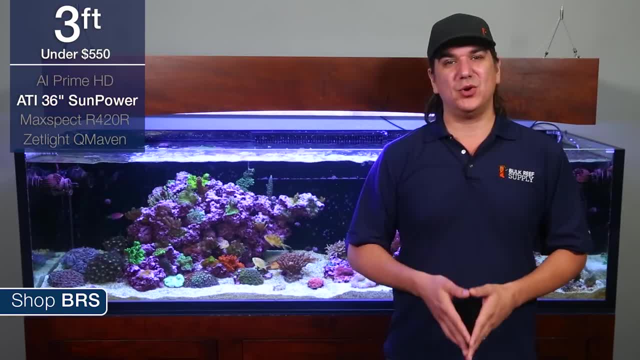 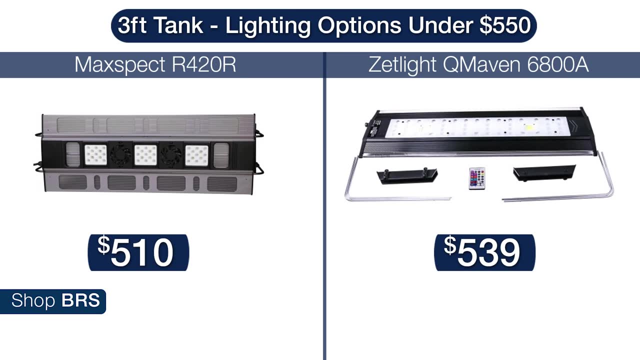 the range of corals you can maintain and again has a plug and play approach to simplicity. As a matter of fact, I think it is a tie between the Maxpec Razor and a Zetlite QMaven 6800A, both of which are more affordable: fixture type lights at just over $500.. The features: 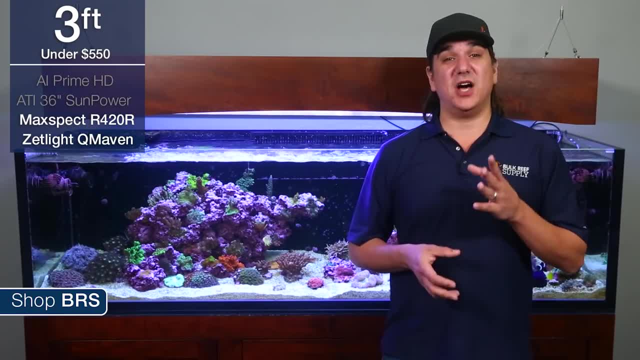 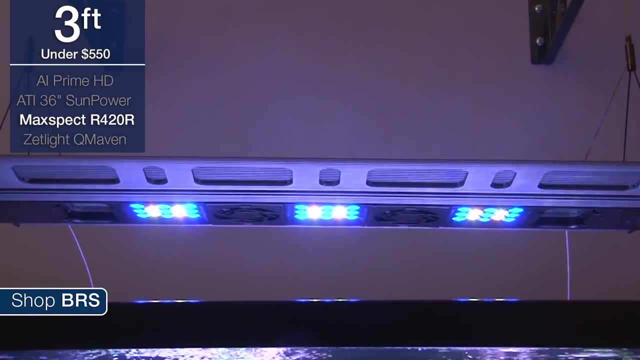 list and build quality is not as solid as the higher end competitors, but dollar for dollar, as concerned to light output, they are a solid value. The Maxpec has three light pucks with 180 watts of LED output. The three pucks will certainly spread the light more evenly over a 3 foot area. 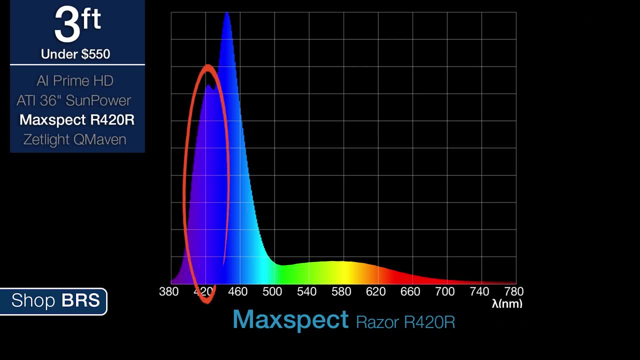 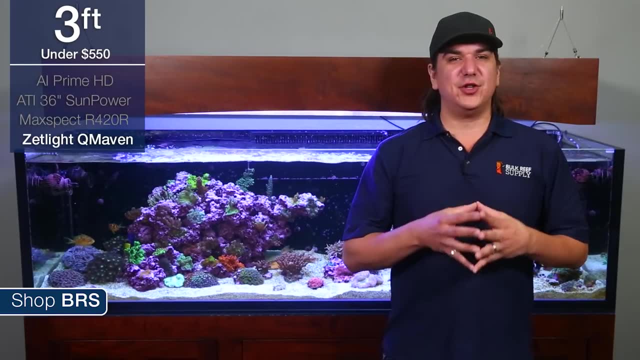 Maxpec includes some unique LEDs in the blue spectrum which a lot of reefers particularly like because they bring out that pop they are looking for with their corals. The QMaven uses a different design which even further spreads out the light. The design: 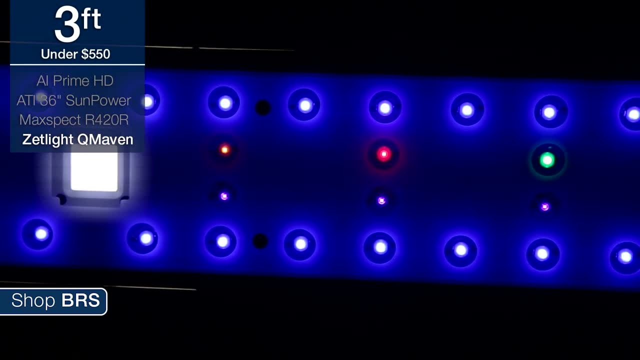 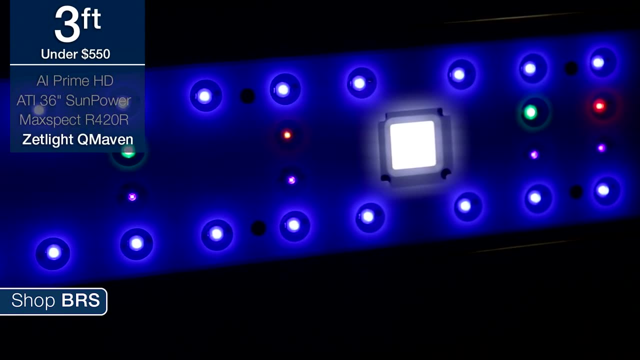 uses two large, dense white LED clusters and then spreads out a large array of 8 violet, 30 royal blue and a few green, red and orange LEDs, for a total of 230 watts. This is the widest of the three options, which will help the light reach areas that would otherwise. 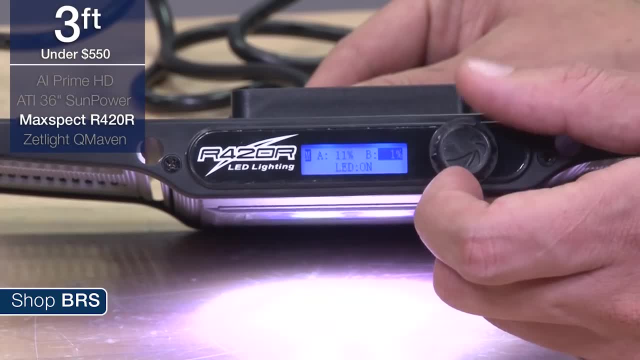 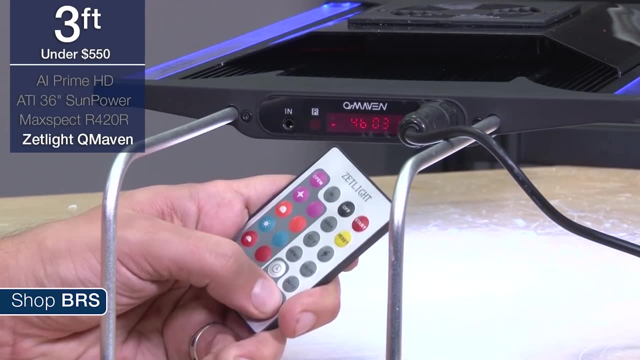 be shadowed with more compact light sources. The controllability of the Maxpec Razor is done via an onboard knob and the Zetlite uses an included remote and it is apex ready to be controlled by an apex controller if you would like. Both of these fixtures have a leg option included or can be hung from the 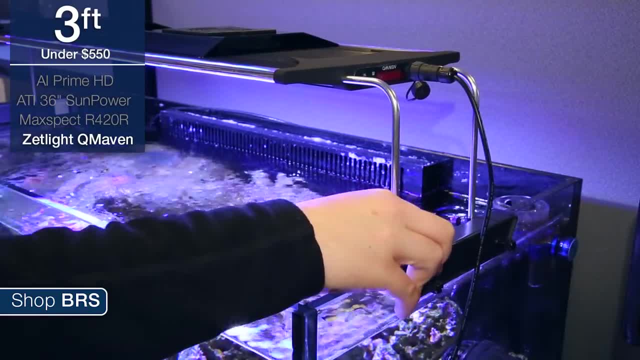 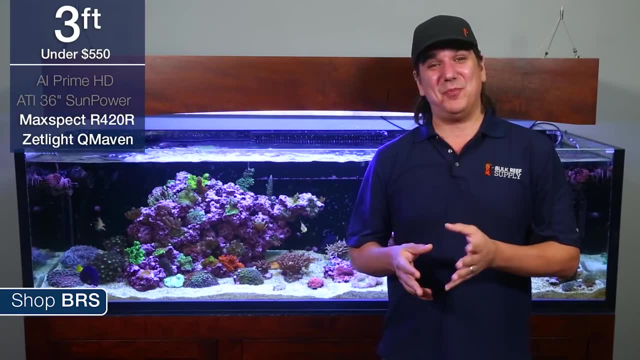 ceiling or wall. The included leg option alone will make these lights pretty attractive to a lot of reefers. I am not going to pretend that either of these options give the impression of being American or German built, and some components are kind of flimsy. but if $500 is about your budget, 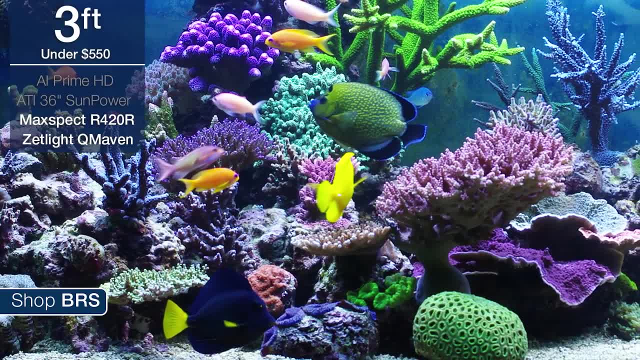 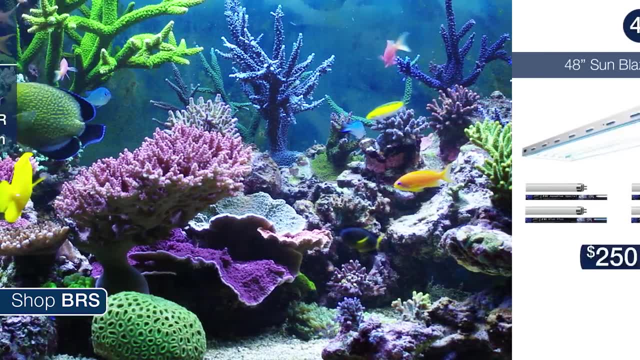 range. both of these options are probably your best bet, Particularly if you would like to bridge that gap between low to moderate light corals to something capable of supporting higher light or demand corals On a 4 foot tank, we are commonly looking at 75,, 90 to 120 gallon tanks. As to lighting, 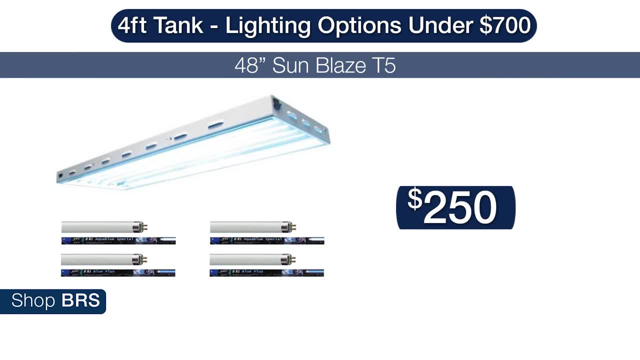 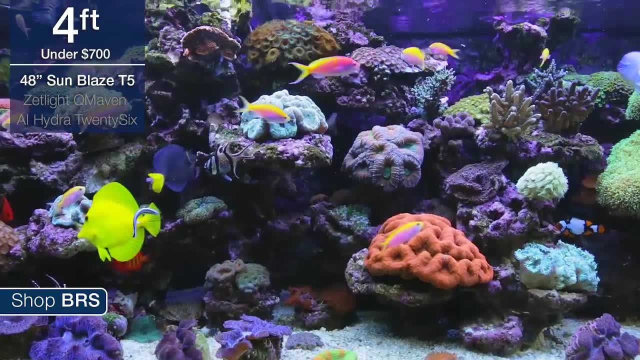 this time I am going to try and stay under $700.. I have to go back to the Sunblaze with a 4 bulb with bulbs for $250.. You can keep a vast array of moderate light corals With a 6 or 8 bulbs in around 3 to 450. you can keep almost any coral you want. Again T5's. 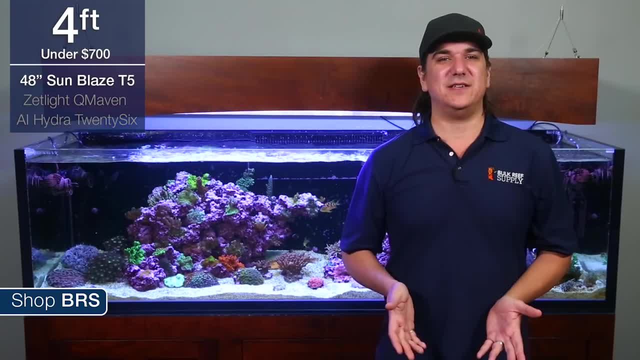 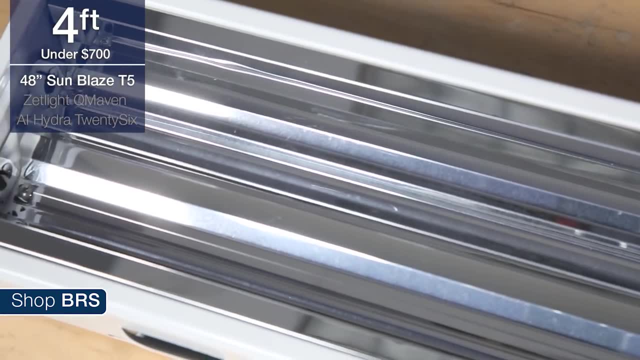 being simple plug and play technology. You can get a lot of light with a 4 foot tank. However, a quick reminder: the Sunblaze's might not last as long and the reflectors are not as optimized as popular brands like ATI, so you need to have appropriate expectations. 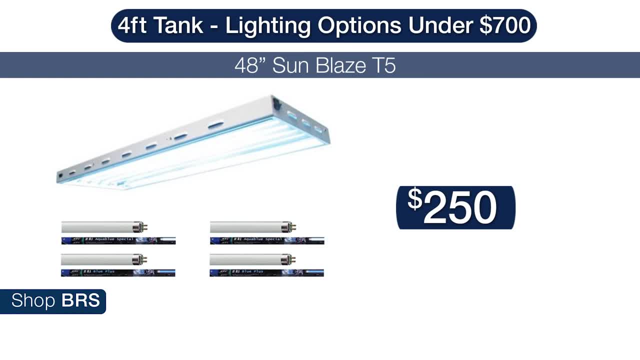 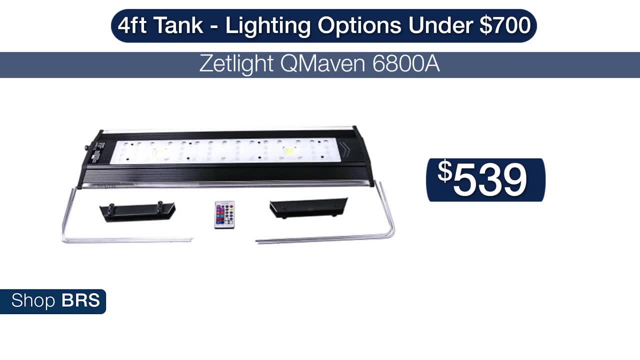 but they are like a half to a third the price and they will absolutely represent value to reefers trying to do this without breaking the bank. Right behind that, at $539, is the same zet light Q-Maven 6800A we recommended on a 3. foot tank Claims to cover a full 48 inch tank as well. however, the sides of the tank might likely be a bit bigger. I don't think there is a lower cost way to buy a 230 watt fixture with this wide of coverage. Similar to that, you could still consider the larger Maxpec Razor which is 43 inches wide. 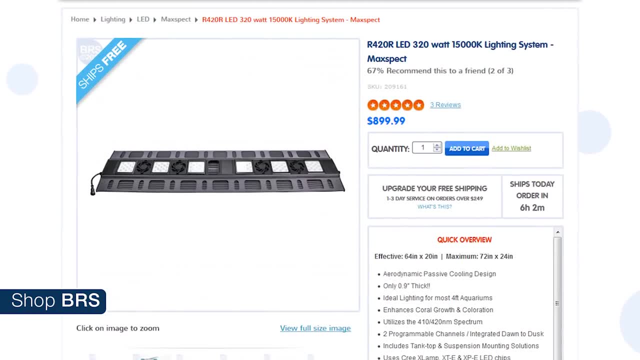 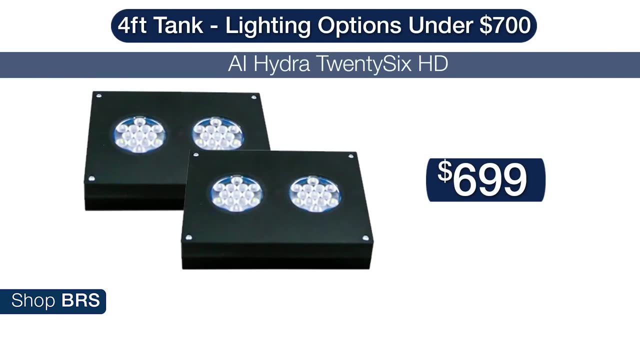 and will cover a 4 foot or larger tank. However, this larger size now has doubled the LED pucks with 6, and is just shy of $900, which is outside our range today. Two Hydra 26's for $699, I think, might end up being what a lot of budget conscious reefers. 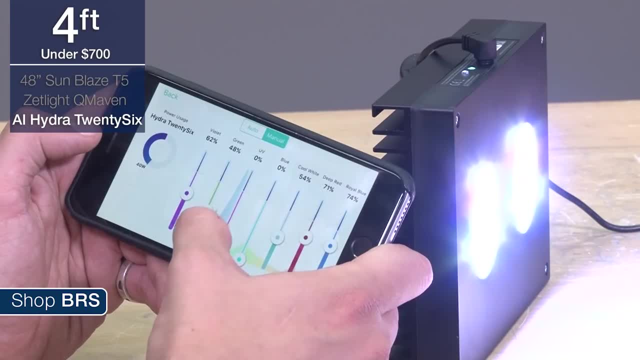 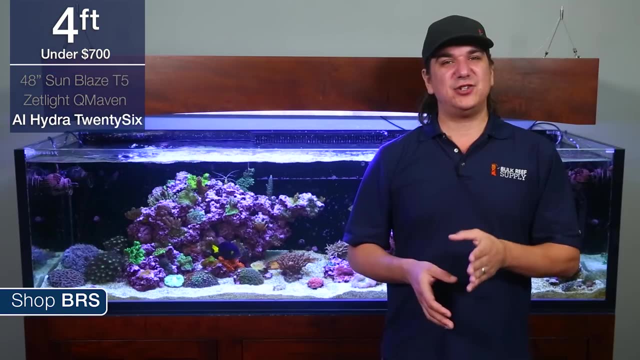 go for in this price range. They are substantially less expensive than the Hydra 52's And if you have a softy LPS or polyp tank you are likely not going to even use half that power anyways. The Hydra 26 is just a much better option for a lower cost tank implementation.